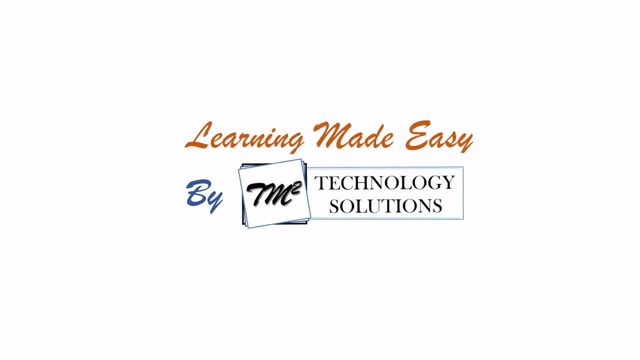 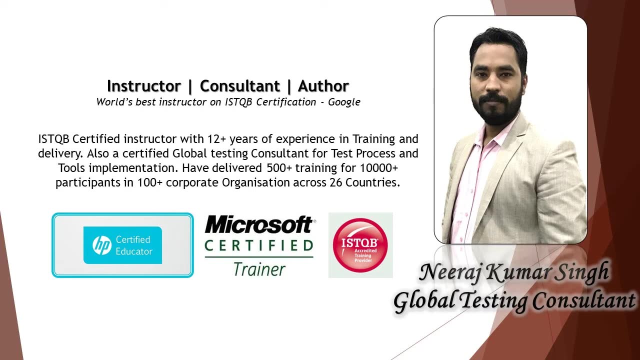 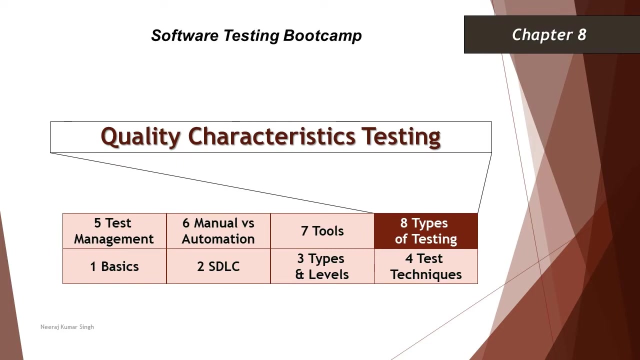 Hello, friends and greetings for the day. Welcome back to another tutorial on our software testing boot camp, where we are talking about the fundamental concepts of software testing, and we are in chapter 8, talking about the quality characteristics testing, and that's where we are continuing ahead with our next segment, which is 8.4, security testing and 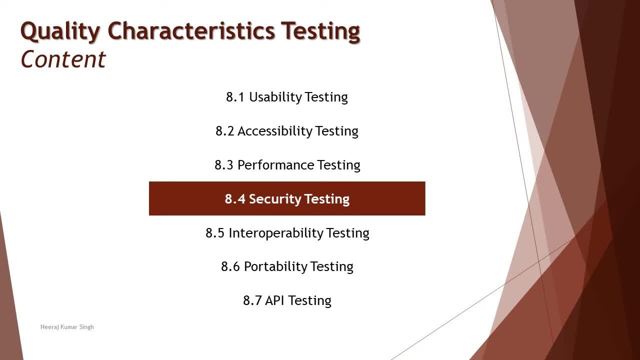 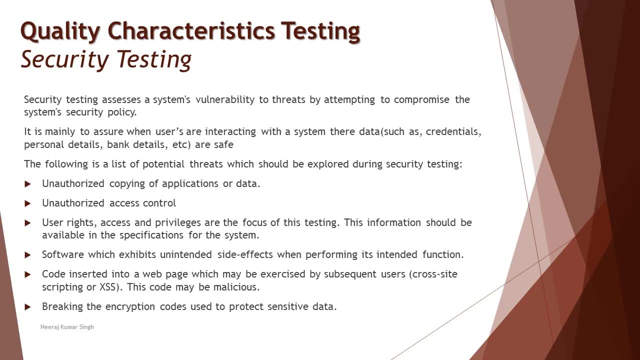 today we'll be understanding what the security testing is all about and how does that help an organization, a test team, achieve a great security. To talk about the security testing, I must first introduce that what kind of security threats we are talking about and by testing them we are trying to eliminate. 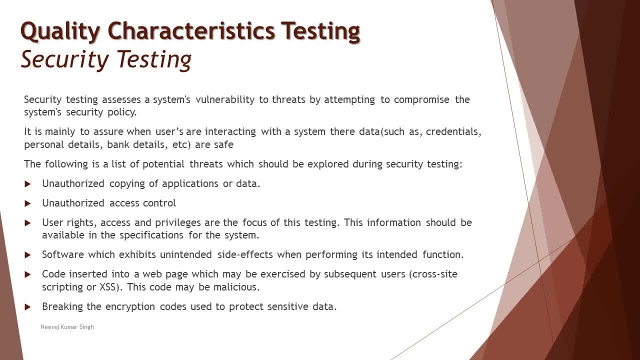 before it reaches to the end user or when it goes to the market. Now, security testing basically assesses the various types of system vulnerabilities to threats by attempting to compromise the system security policy, and this, in simple terms, generally means there are a lot of vulnerabilities which may be impacting the system data, which is highly secured in terms. 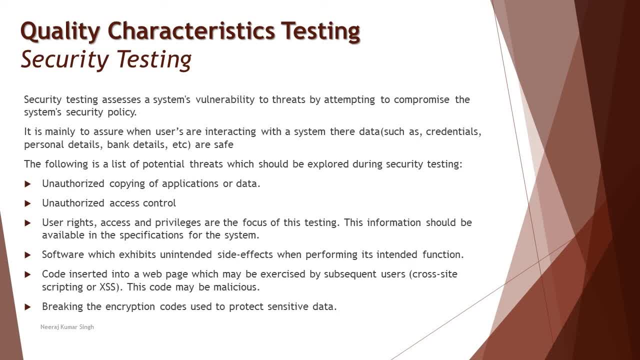 of you, but of course, there might be various ways by which it can be penetrated through and an external person can hack into your information and retrieve all your personal details or data which you might be thinking is pretty much secured. So today we'll be understanding about. 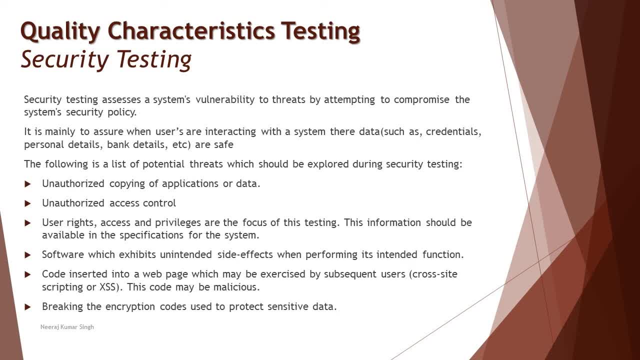 the same that how security testing looks forward to these threats and what can be done best as an approach from testing point of view to perform this on a very high level. So it is generally. if there is a definition to security testing, it is mainly to secure your data when you're working on. 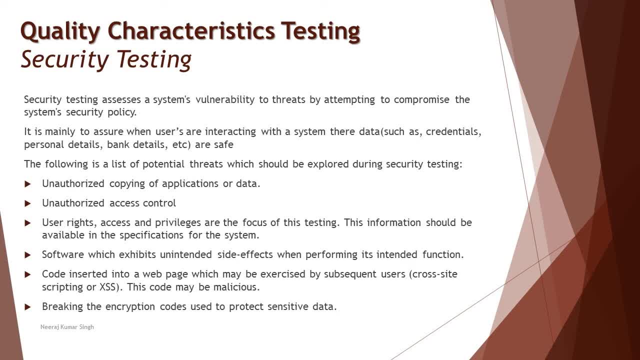 any system or any platform. It is mainly to assure a user, when user is interacting with a system, that the data, whatever the data could be, it is about your credentials. it could be about your personal details which you might be securing there and including any other platforms when you're talking. 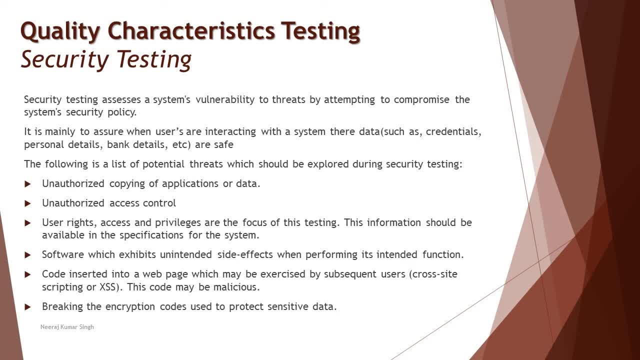 about your one-time passwords. you're talking about the bank details On a network, so you just make sure that these data are safe when you're using a browser, when you're using a particular platform, operating system, etc. So there are many ways by which this can happen. so we are trying to understand, with a small list here, that the following is a. 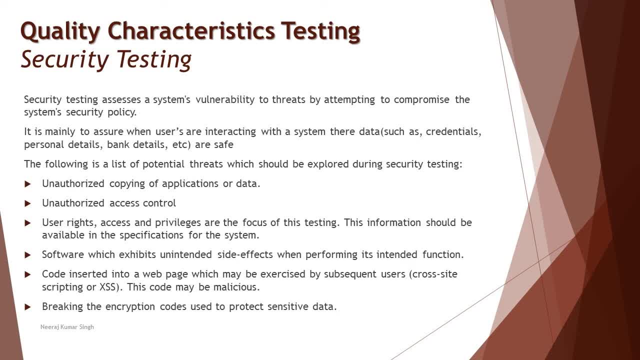 list of potential threats which should be explored during security testing. So, generally, a security testing team is well specialized and well trained on how to measure these parameters in terms of threat to reduce the security problems, security breaches on an application or in any particular platform. So these are some of the examples of potential 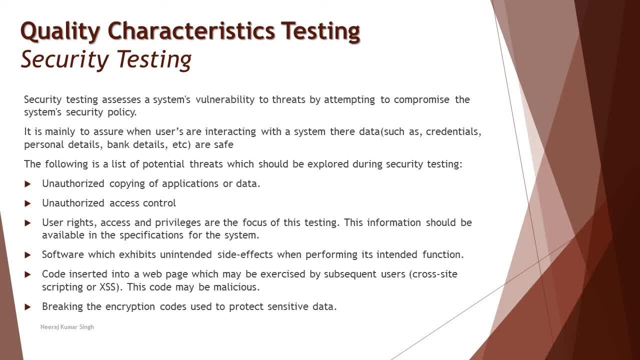 threat which can be exposing your secure data to the people, and that's what you call it as the security breach or leak of the data. Now, unauthorized copying of the application or data, which is a very simple and straightforward thing to be involved in, is a very simple and straightforward thing to be involved in, is a very simple and. 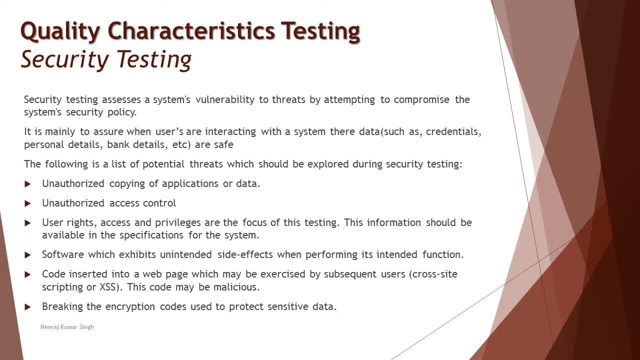 that when you try publishing certain content with a copyright symbol on top of it, it means that the other people do not have any rights of claiming that that content belongs to them. They can always use it under the fair use policy because the company might have allowed other. 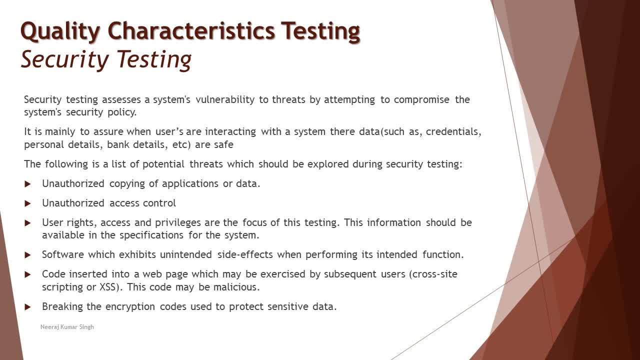 people to make use of it as a reference for study purpose or for presenting purpose. but you have to make sure that if it is having a fair use policy associated with that, but unauthorized copying of any application or data is also a security breach or it's a threat. Talking about the unauthorized access control, that means you do not have the 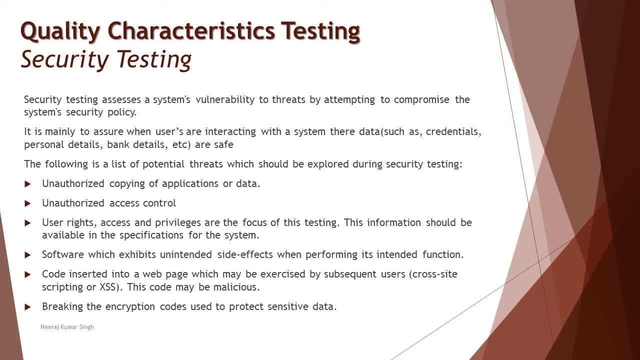 right parameters to log in into an account, but you are trying in different, other ways by which you can break through the login credentials. Also, user rights, access and privileges are the focus of this testing, which checks whether what kind of authorization you give through different portals, including your browsers, including saving a password. Did you know that? 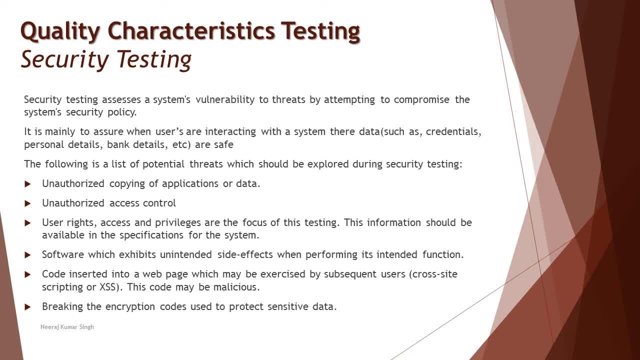 saving a password is not so safe for you because if, in case, any user can penetrate into your browser, they can very well retrieve all your passwords. So it's not so safe to even save your passwords over the browser, rather prefer making a note of it in a diary, in a notebook, outside the computer. 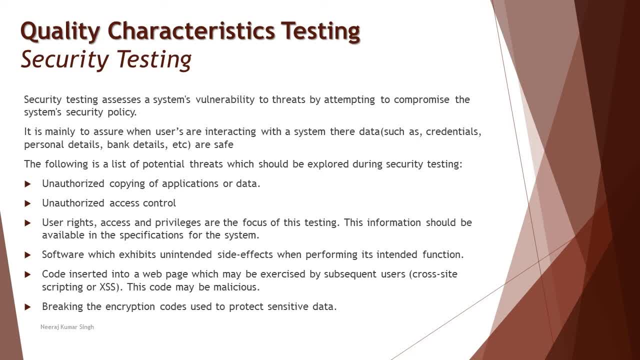 which is pretty much more secure. Anyways, if you're deep dive, you're going to have to make sure that you have a password and you have a password and you have a password. even that is not secure. User rights, accesses and privileges are the focus of this. 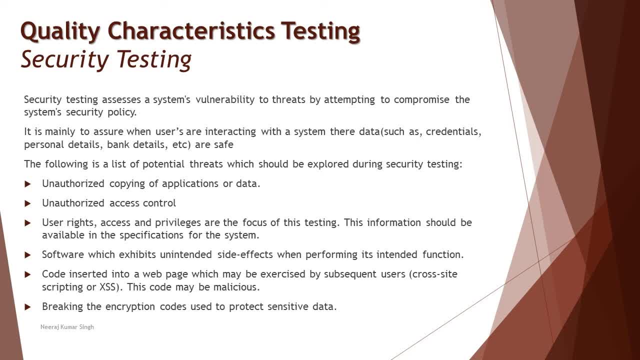 testing. This information should be available in the specification of the system that how this is going to happen. The software which exhibits unintended side effects when performing intended functions. The intended functions are basically the main thing, what a system should do, but if in case, it is doing anything like different than usual, and that's where we can understand that. 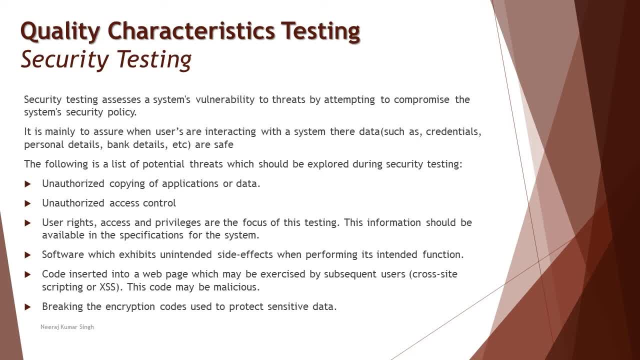 as a threat. That means this application was not supposed to do something on its own. So generally the activity log are kind of like a notification which says that hey, somebody tried, you know, accessing your account in this location from this IP address which is trying to prevent your security. 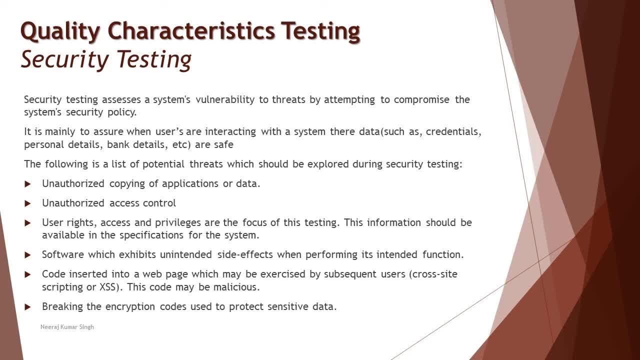 breach right and you get notified and you have to take necessary actions immediately to change your password. Also, code inserted into the web page which may be exercised by subsequent users which could be used as a threat to your account. So, if you have a password and you have a password. 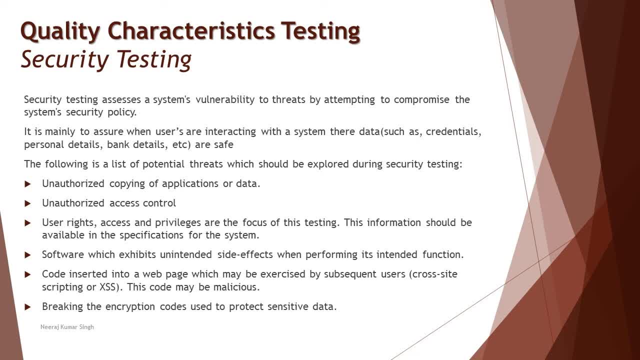 which could be the cross-site scripting or XSS. this could be malicious also. So it's more about like kind of like installation on a pop-up which appears just from nowhere and you agree to install that or agree to download a particular file which may trigger any kind of malicious code to be 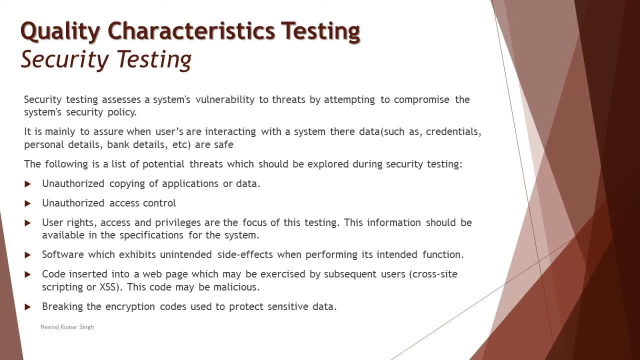 installed on your system or on your browser which may help them to hack your data, Also breaking the encryption codes used to protect sensitive data Encryption code. Generally, we know that our passwords are not displayed as we type them. It is always masked with some asterisk and there's an encrypted value behind the screen which the system 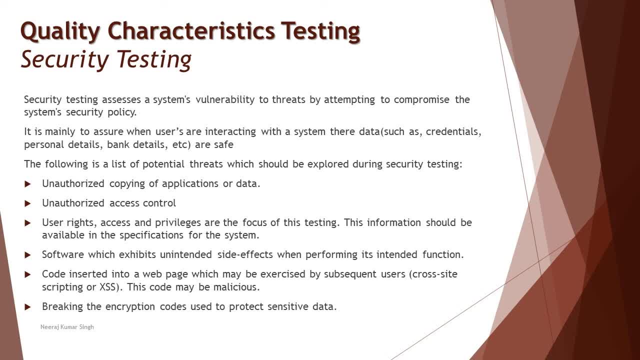 captures to make sure that right there, when you enter the value, it is encrypted in a way that it does not let anyone find out what exactly was the password, even if anything wrong happens. But people are trying to break through the encrypting code. So if you have a password and you have a 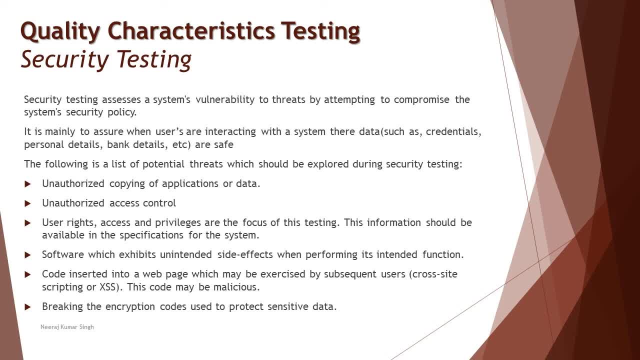 password. you can use the encryption code itself to see and retrieve back what password was entered. So there are such things which are happening around. So just make sure that try to not save the browsers, save the passwords on the browser, because if in case somebody can decrypt it, then 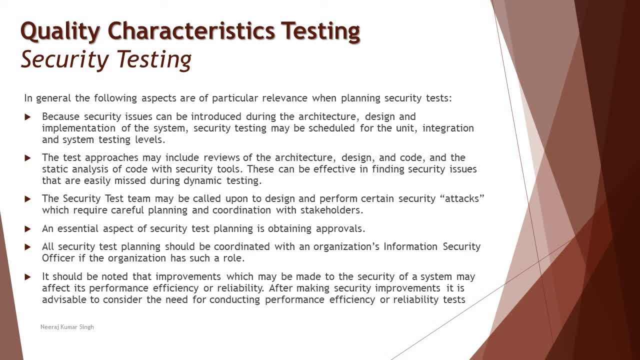 you are still not safe. On the other hand, talking about what a security testing team should do or what a security team generally takes care of in order to measure the security threats and prevent it to happen, How does the security testing generally takes place? So, in general, the following aspects are: 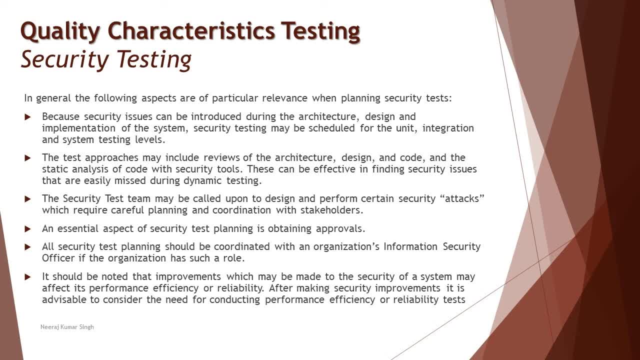 of particular relevance when planning for the security test. Now, in an organization, we will have a separate team who's going to be responsible for performing all necessary security tests. It's not the same tester who was doing unit testing or integration testing. We completely have an. 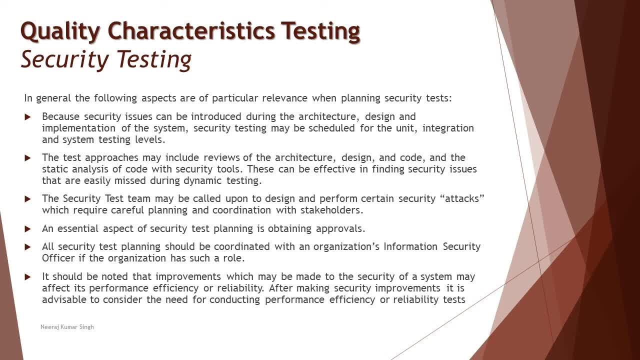